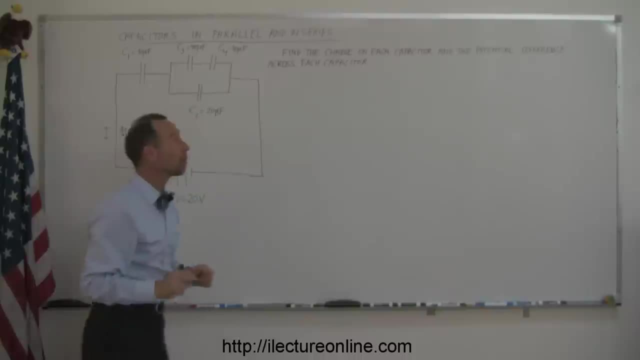 the more correct way of saying that, because typically, when we measure the voltage or the potential difference, we take a voltage measurement device called a multimeter and we actually measure the voltage across the terminals of a capacitor, so that's why we use the word across. Okay, how do you do that? where do you start? Well, you do the same thing, like what we. 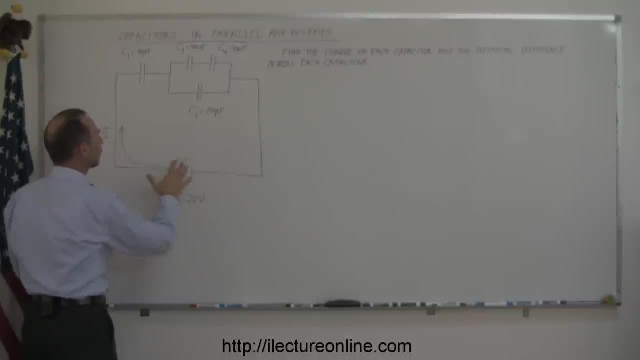 did before. for a moment, you ignore that. the battery is there. you know it's there, but just ignore it. excuse me, you're going to now find the equivalent capacitors in stages, so, just like before, you're going to start by taking these two capacitors right here and turning those into a 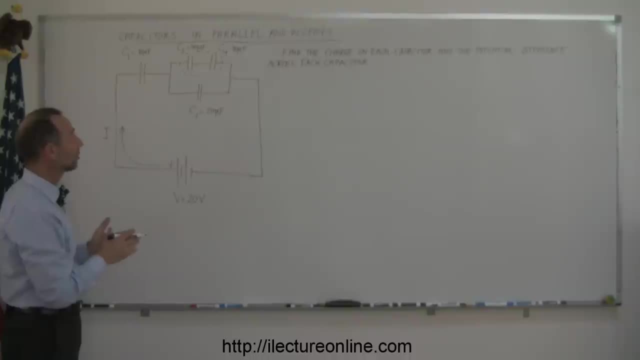 single capacitor. of course those two are in series. since they're in series, you need to find the total 에서도격 제아 화omeoh strand in series. you need to find the totalicker vindh spot at RBrCa and capacitance by taking the product over the sum. and of course this is capacitor 3. and 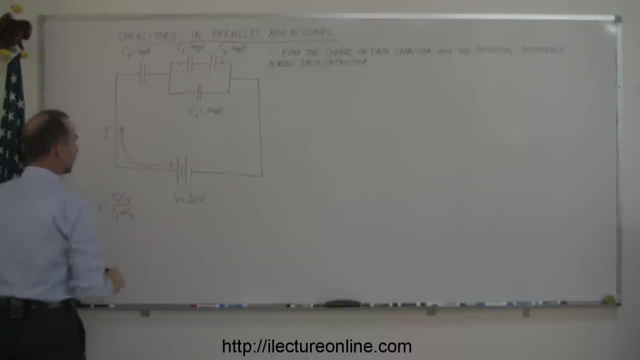 capacitor 4 divided by C3 plus C4. So we find that by taking the product over the sum, So in this case that's 40 times 40 divided by 40 plus 40. And, as you will notice here, the answer here is 1600 divided by 80, which is equal to 20.. So it turns out, when you have 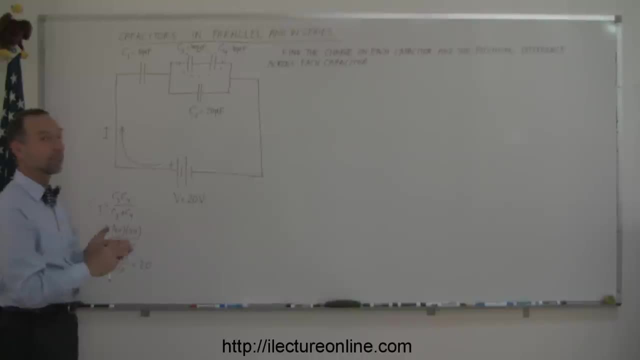 two capacitors that are the same size in their series, the equivalent capacitors will be half that value, so 20 microfarads. So this whole circuit can now be replaced by the following circuit, which is this one. here We still have the original 10 microfarad capacitor. We now have 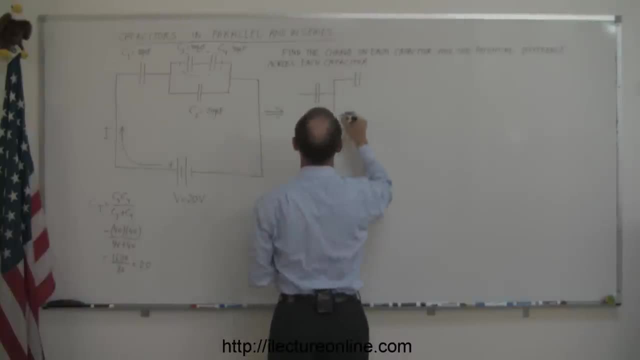 our parallel circuit. but these two combined now will turn into a 20 microfarad capacitor. This one is also a 20 microfarad capacitor and now we have this equivalent circuit. Plug in the values, we have 10 microfarads. 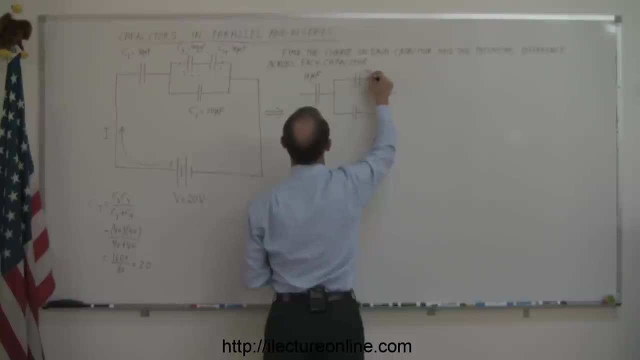 Here: these two now will become a 20 microfarad capacitor, and this is still your 20 microfarad capacitor. So notice: the only thing you've done is taken the top two here and turned into a single capacitor. We continue now by taking these two capacitors right here and 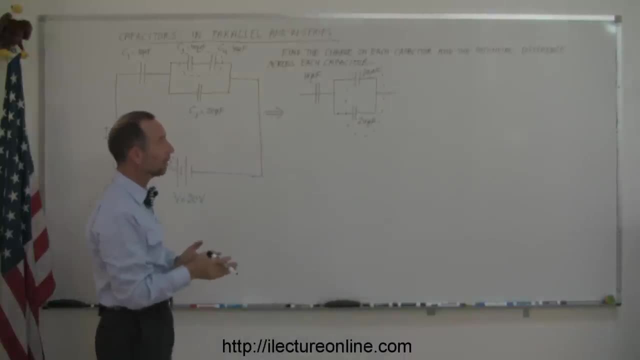 turning them into a single capacitor. In this case they're connected in parallel, Capacitors connected in parallel. you simply add them together. So C total equals C1, or well, whatever you want to call it. Well, whatever they are, instead of C3, 4 combined in C2, hmm well, we'll just in general. so C1 plus C2, so this is equal to that. could confuse you right. So let's call this C3, 4.. That's the combination of 3, 4 together added to C2, so it would be equal to 20 plus 20, which is 40 microfarads. So those two combined turn into a single capacitor of 40 microfarads. 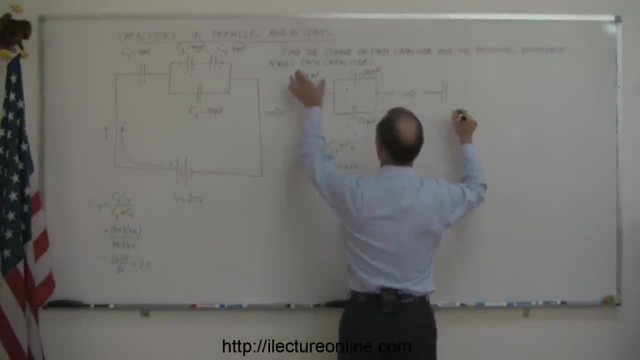 And And. if we then draw this over here, we still have our original 10 microfarad capacitor and these two combined now will become a 40 microfarad capacitor. That's our 10 microfarads. So we still have C1, right, This is still C1. It hasn't changed C1.. And this now becomes C1,, C2, C3, and C4 all combined. so we call this C2, 3, and 4 all combined into a single equal capacitor. 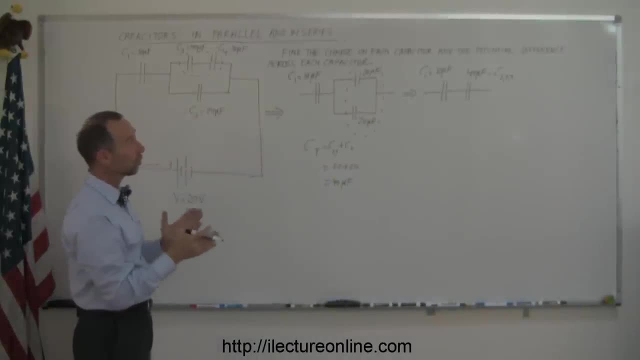 So now the next stage is to take those two and turn those into a single capacitor and of course, since they're in series, the total capacitance is equal to the product. that would be 2,, 3, and 4,. there we go, divided by the sum C1 plus C2,, 3, and 4, like that, So that would be 10 times 40 over 10 plus 40, which is 400 microfarads. 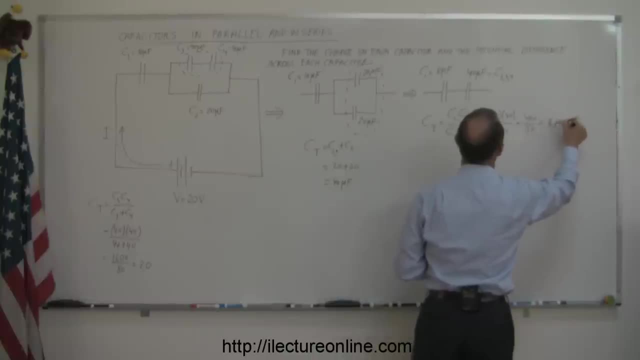 Over 50, which is 8 microfarads. So this whole circuit could be replaced by a single 8 microfarads, which is considered the total or equivalent capacitance hooked up to our battery. Oop- too many lines here. Our battery and our battery is has a potential difference of 20 volts. 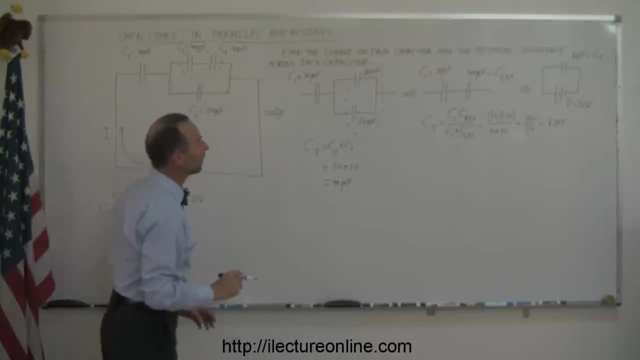 All right. So now what we've done is we've taken our circuit We had before hooked up to a 20-volt battery, found the equivalent capacitance in stages until this whole circuit right here could be replaced by a single 8 microfarad capacitor, still hooked up to our 20-volt battery. 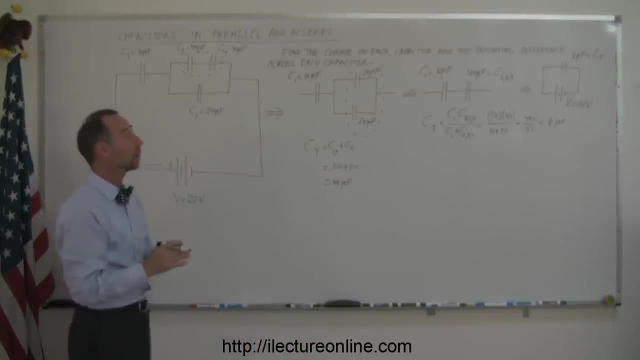 All right, So that's what we have learned so far. but now can we go ahead and answer the questions? find the charge in each capacitor and the potential difference across each capacitor. So, looking at this situation, we have a single capacitor now hooked up to a 20-volt battery. 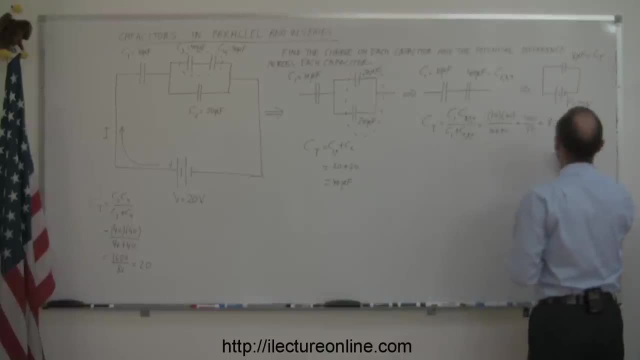 We can then say that the potential difference across this one. so we can say that C total or the voltage across C total. So the voltage across C total is equal to 20 volts. The capacitance of C total. C total is equal to 8 microfarads. 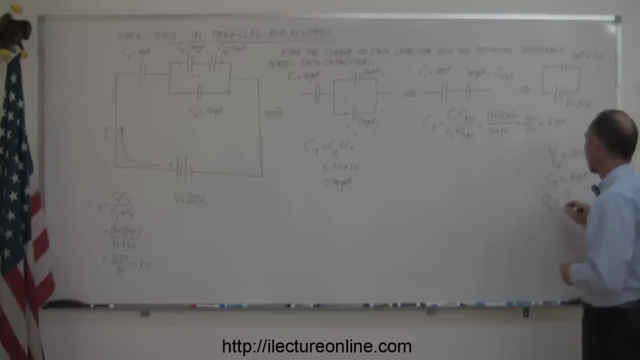 So then, how much charge is on C total? So charge total, how much is that equal to? So we have to go back to the equation that tells us the difference, The definition of capacitance, and that equation says that the capacitance is equal to the charge placed on a capacitor divided by the voltage that pushes us there. 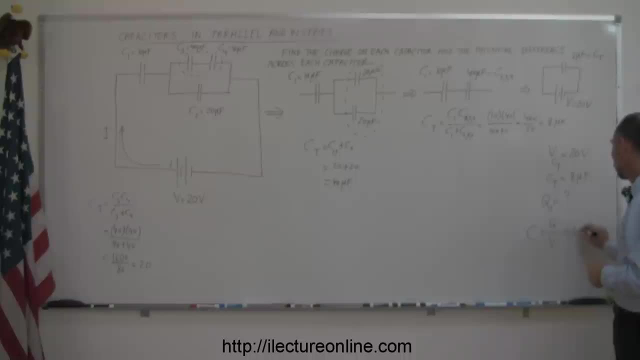 So if we want to solve this equation for Q, we can say that Q is equal to C times V. So to find the charge on this equivalent capacitor we simply take the capacitance and multiply it times the volts that push the charge on there. 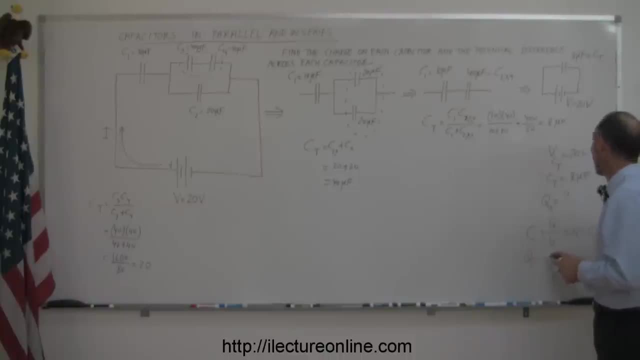 So in this case Q is equal to C times V, which is 8 microfarads Times 20 volts, and that would be Q is equal to, and of course that would be Q total on the whole circuit is equal to 160 microcoulombs. 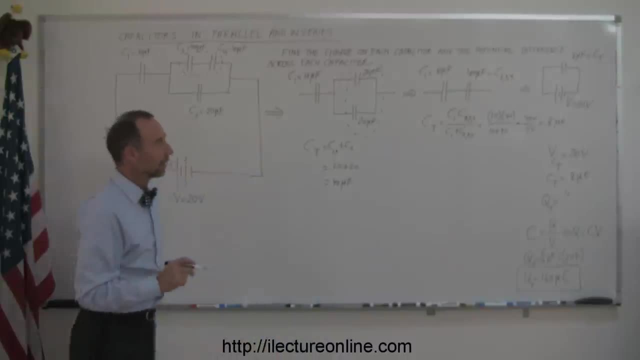 There. So we determined that if we take this entire circuit and replace it by a single equivalent capacitance, the charge on that single equivalent capacitance would be equal to 160 microcoulombs, saying there would be 160 microcoulombs of charge placed on the circuit. 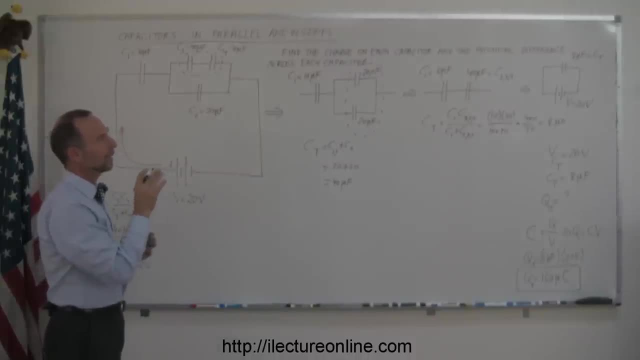 All right, but now how do we find the individual charges on each capacitor like that? All right. for that we have to follow the following rule: If capacitors are connected in series, the charge on each is the same as the total charge on the equivalent capacitance. 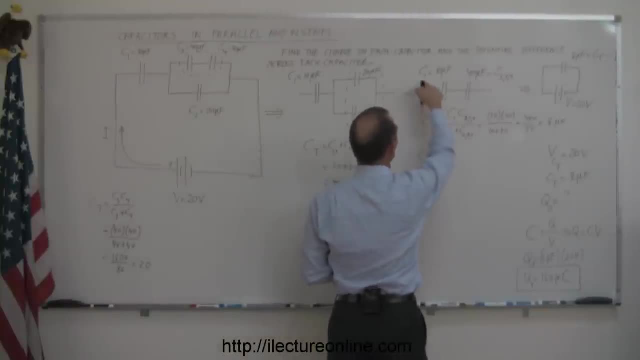 All right. that means that the charge on capacitance one has to be equal to the charge on the equivalent capacitor two, three, four, which means this is the equivalent capacitance by combining a capacitor two, three and four together, and that has to equal the total capacitance that we found right here, which means that the 10 microfarad 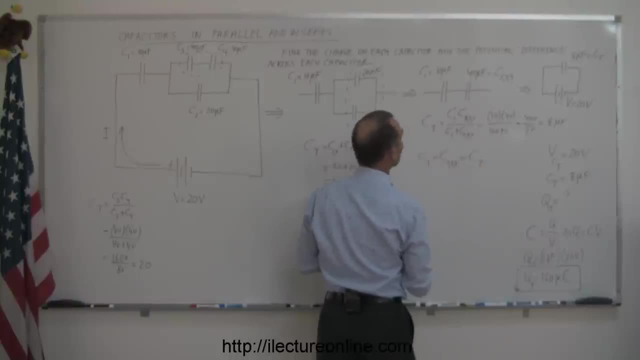 capacitor has 160 microcoulombs of charge on it and the 40 microfarad capacitor has 160 micro coulombs of charge on it, and you might say how that is that possible? if the total charge is 160 microcoulombs, shouldn't, like each have maybe half or a portion of it so that it adds up to 160? 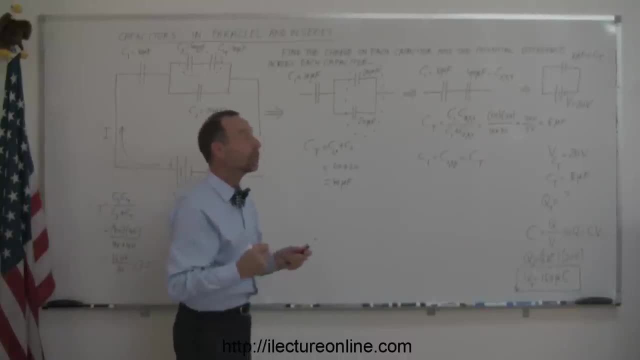 and the answer is no when they're connected in series. what that means is that whatever charges you place onto this particular capacitor plate causes an equivalent amount of charge to be pushed away from the other side of the plate, which then runs down or flows down. i guess they don't. 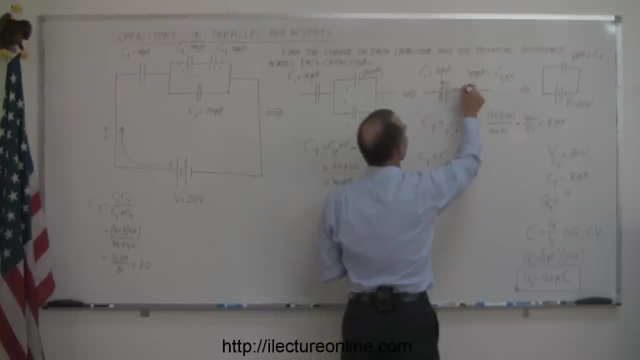 run. charges don't run. they flow through the you to the conductor and they'll deposit these charges on this side, which then will push away the positive charge on the side, making that negative, and you can see that it. it kind of the charge just kind of goes from capacitor, capacitor, capacitor, placing the same amount. 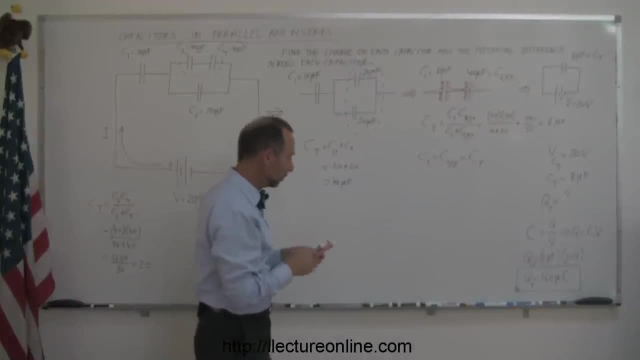 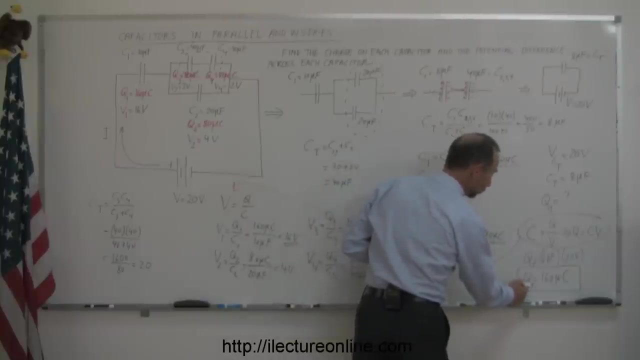 of charge in each capacitor in a series circuit, which means that all these capacitors will have 160 microcoulombs of charge. and we just looked at this and we realized i made a mistake- and it's easier to do on a problem like this, this complex. i found that the total charge was 160. 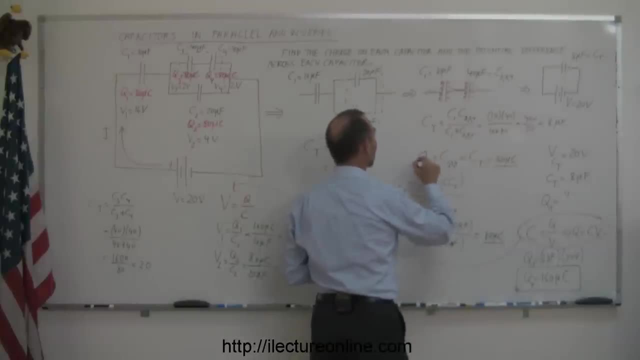 microcoulombs and what i have here this should be: the charge on one is equal to the charge on those, which is equal to the total charge. this is a charge and not capacitance- equal to a 160 microcoulombs. so just to make sure, i was talking about charge there and not about capacitance. so hopefully that 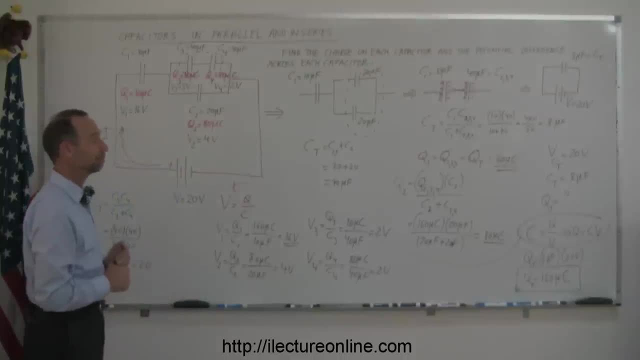 might clear up just a little confusion that i might have created by that error, which means going back to the original circuit. so i'm going to have to do a little bit more work on this one because i'm- since C1 here is the same as this C1 there. 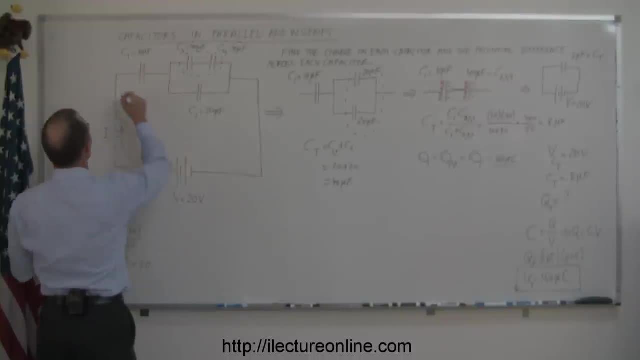 this one here has a charge Q1, equal to 160 microcoulombs. Yep, I said the right thing, And that means that this also has 160 microcoulombs of charge on it. All right, so then I go over here and say: 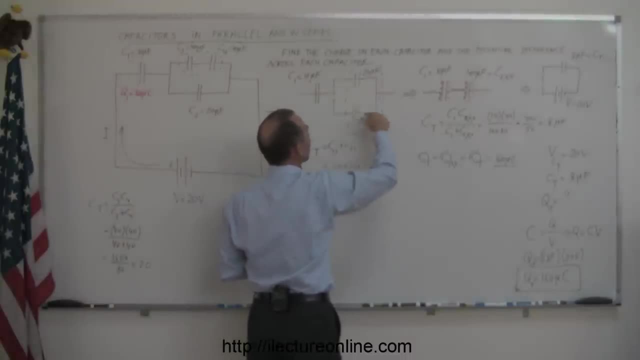 how is that 160 microcoulombs of charge distributed across these two capacitors? Well, it turns out that since the two capacitors are equal and they're parallel in parallel capacitors, the charge is distributed across them according to their size. 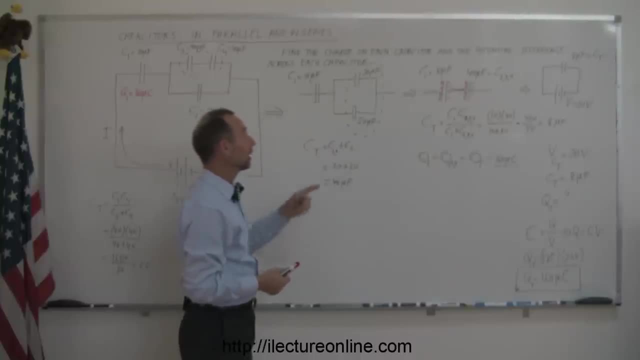 Since they're equal size, they will get the same amount of charge. If this one happened to be twice as big as this one, it would carry twice as much charge. So what we can say is that the charge on this one is equal to the total charge on the two of them. 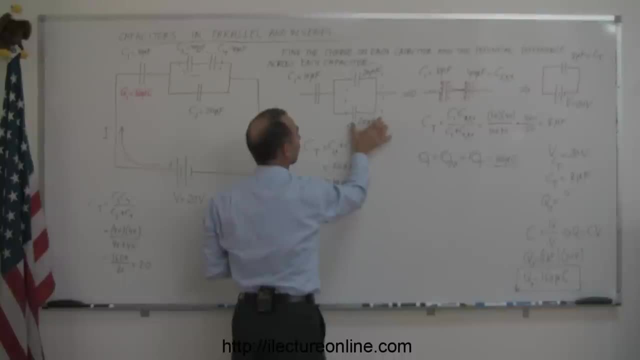 times the charge on this one, So the capacitance of this one divided by the total capacitance. So what I can say here is that the charge on the second capacitor is equal to the charge on the sum of the two, so Q2 plus Q3, 3, 4.. 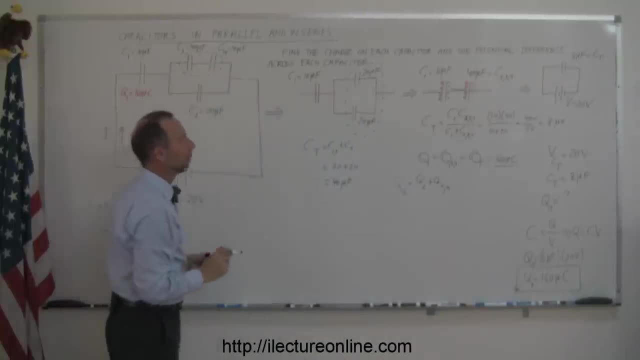 So that would be. this capacitor is really the sum of those two, right? So the charge on Q2 would be the charge on both of those, And that's really not the right way to say it. Let me go back. The best way to explain that one is: 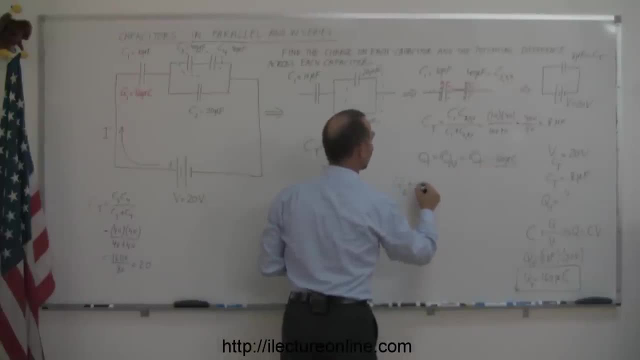 it stakes the 160 microcoulombs. so that's equal to the charge on the three combined. like that That's a better way to say it: Multiplied times the size that's charge on those two. multiplied times the size of the second one. 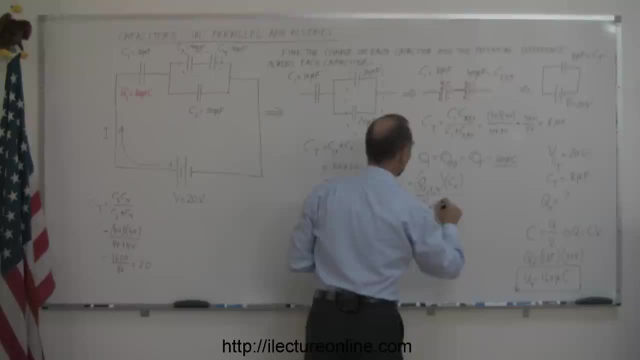 divided by the size of the sum: C2 plus C3, 4.. That's a better way to write it. So let me explain what I just did To find the charge on this one. here you take the total charge of the distributor on those two. 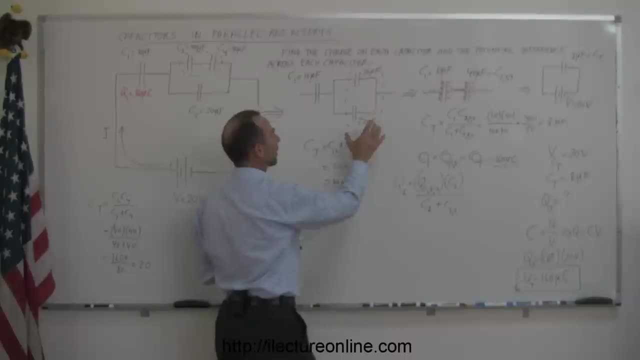 which I say is Q2,, 3,, 4,. right, You multiply it times the size of this capacitor C2, and divide it by the sum of the capacitance. like that, So put it into practice. This is equal to 160 microcoulombs. 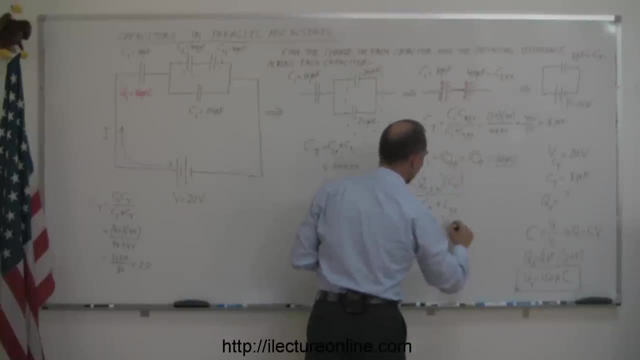 times the size of this capacitor. right here that we want to find the charge on 20 microfarads divided by the sum of the two, which is 20 microfarads plus 20 microfarads. microfarads, right there. 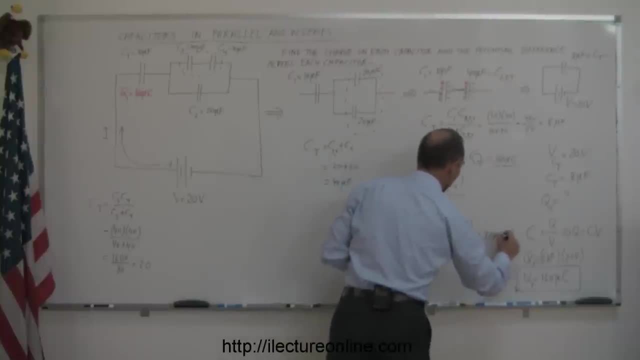 and that is therefore equal to 80 microcoulombs. Just as I predicted, since the size of the capacitor is the same, they will each carry half the charge. That means this one gets 80 microcoulombs and that one gets 80 microcoulombs. 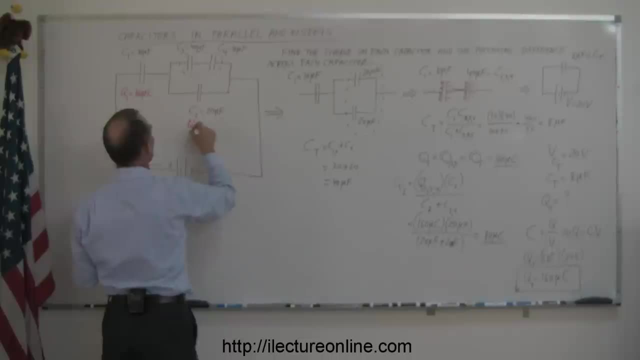 So this one. right here we can say that Q2 is equal to 80 microcoulombs, and those two combined also carry 80, 80 microcoulombs of charge. Now for the last part. we know that this capacitor is really the equivalent. 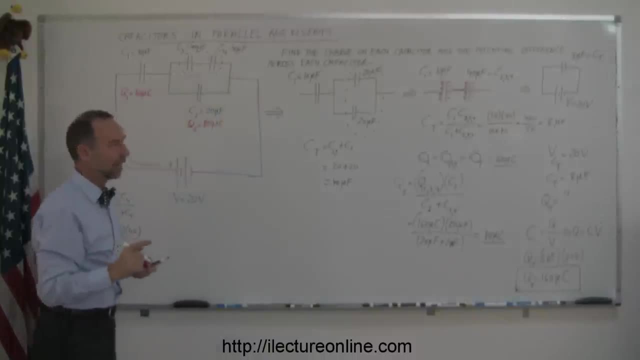 of these two capacitors, and those two capacitors are in series And, just like before, when capacitors are in series, they each carry the total capacitance, which means if the two combined carry 80 microcoulombs of charge. that means each one of them. 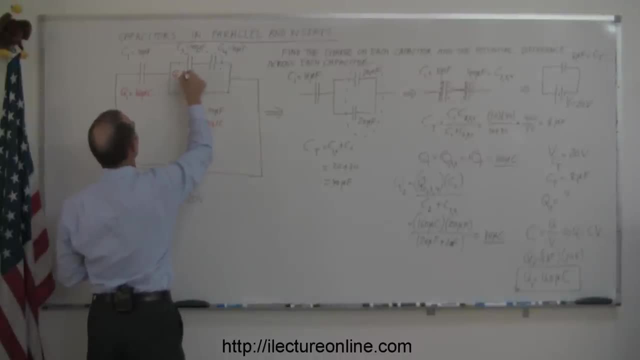 must carry 80 microcoulombs of charge. So Q3 has to have 80 microcoulombs of charge and Q4 must have 80 microcoulombs of charge, And that's how we determine the charge on each of the four capacitors. 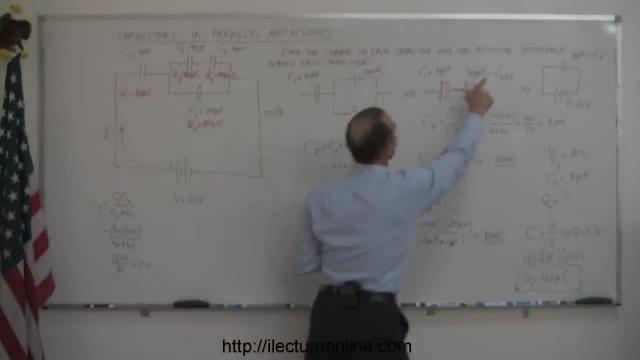 Now the next thing we need to do is also find the potential difference across each capacitor. So, going back to the definition of capacitance, and where do I have that equation Right here, I can then see that I can use that equation to find the voltage across each capacitor. 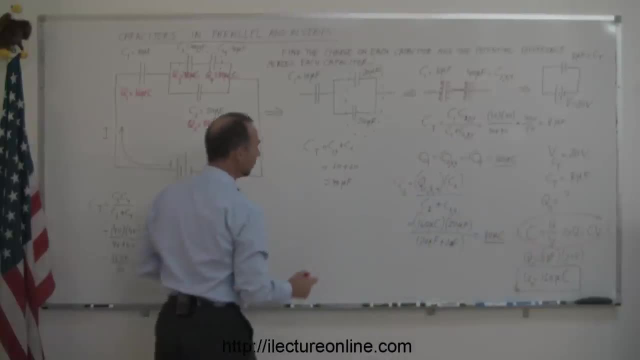 by changing this equation or solving it for V. Excuse me, So we'll take this here and we'll say that the voltage across each capacitor is equal to the charge across each capacitor divided by capacitance, So applying that equation to all four capacitors. 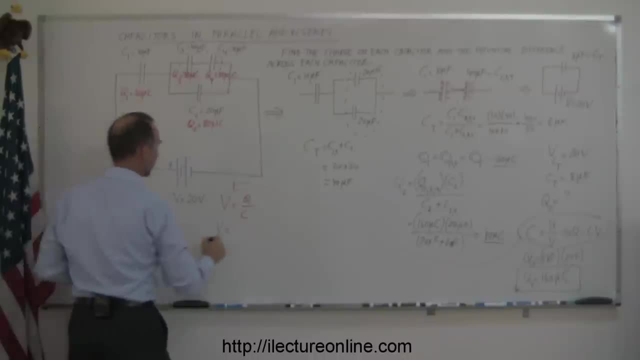 voltage across the first capacitor is equal to the charge Q1, divided by the size of capacitance 1.. So that's equal to the charge which is 160 microcoulombs divided by 10 microfarads, and so that's equal to 16 volts. 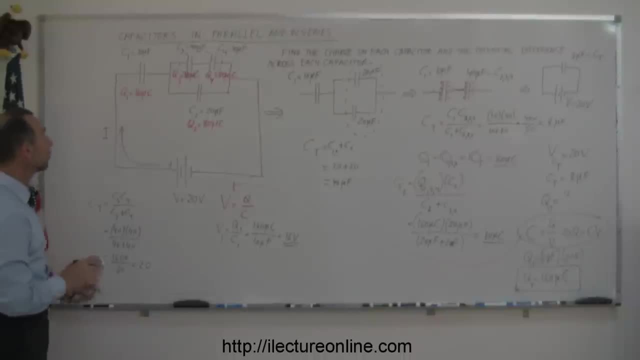 So this tells me that V1 has 16 volts across it. That makes sense, then, to say that if the total is 20 volts and this has 16 volts on it, that this branch right here will have 4 volts on it. Well, we can figure that out. 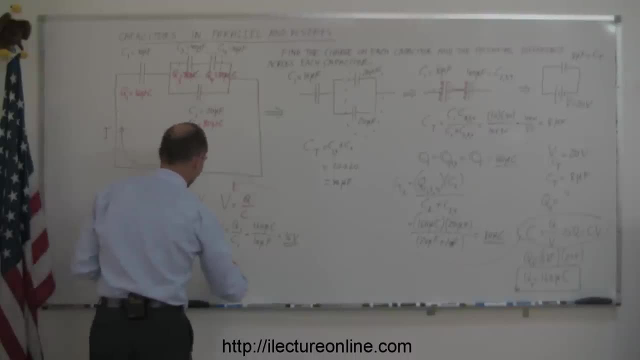 by calculating the voltage across C2.. So V2 is equal to Q2 over C2, and Q2 is equal to 20, microcoulombs. Oh no, not 20, 80.. 80 microcoulombs divided by C2 being 20 microfarads. 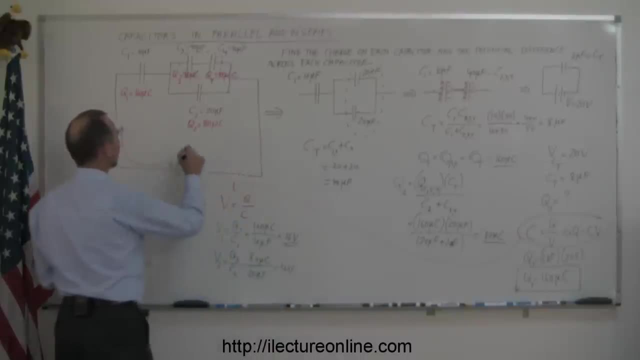 and, sure enough, that's equal to 4 volts. So, just as I predicted, V2 is equal to 4 volts, V1 was equal to 16 volts. All right, Now what about the voltage across these two capacitors? 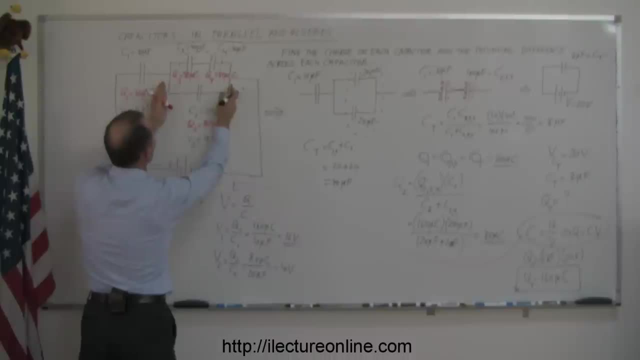 Now, if V2 across these, this one- is 4 volts, it must be 4 volts across this one, which must be split between these two capacitors, and since they're equal in size, I would bet that they each have 2 volts across them. 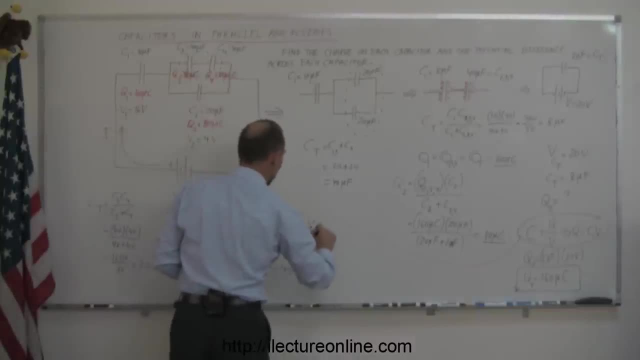 But again making sure we can say that V3 is equal by definition to Q3 divided by C3, and the charge on the third capacitor is equal to 80 microcoulombs and the capacitance of the third capacitor is 40 microfarads. 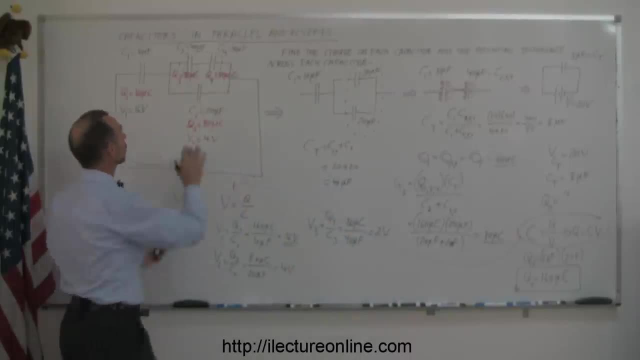 and, sure enough, that's equal to 2 volts. So we can see that the voltage across the third capacitor, V3, is equal to 2 volts, and doing the same for Q4,. V4 is equal to Q4 divided by C4,. 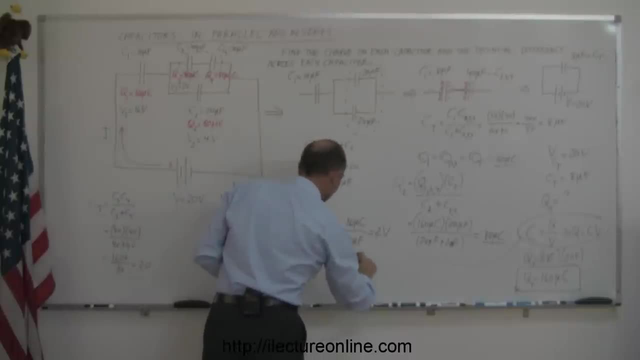 which is equal to Q4,, which is equal to 80 microcoulombs. C4 is equal to 40 microfarads, and sure enough, this one also looks like it's carrying 2 volts, so we can say that V4 is also equal to 2 volts. 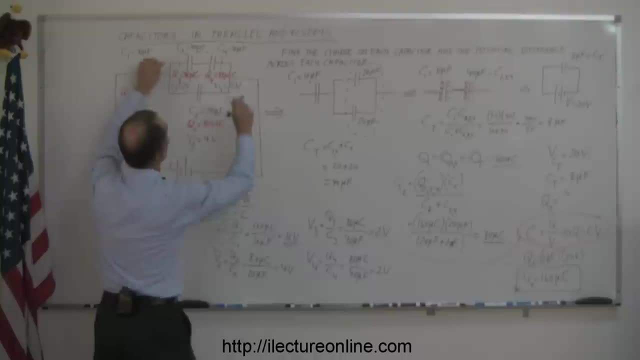 And that makes a lot of sense, because the 2 volts plus 2 volts across this branch must equal to 4 volts across this branch, and then 4 volts plus 16 volts should add up to 20 volts. so it looks like I have the right values. 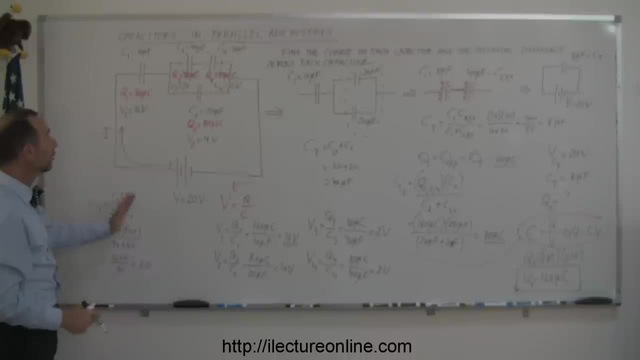 And that's how you solve a problem like this. So again to recap, if you're given a parallel and series capacitor circuit attached to a voltage supply or a battery, you must first find the equivalent circuit until you can replace the whole circuit by a single capacitor.